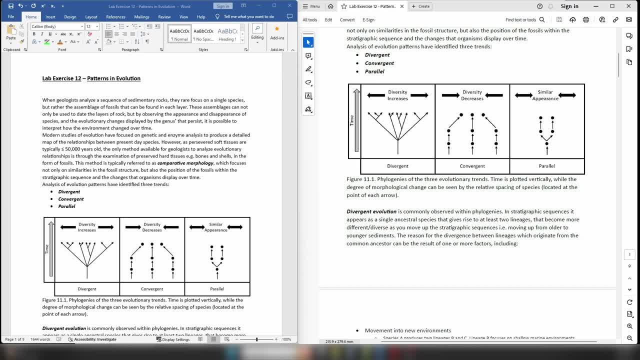 in all cases, they'll look at what kind of sedimentary structures can be seen. So they will then take all this information and they will use it to produce an environment of deposition for each layer or a package of layers. Now we also know that they will relatively date. 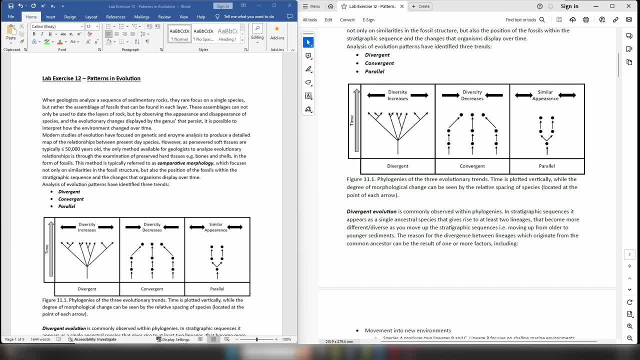 the sequence, so they'll work out the chronologic order for each of the layers, and then they'll use fossils to try and put that sequence in the context of the larger geologic time cycle. Now, another thing that can be done with this sequence, though, is we can analyse the fossils. 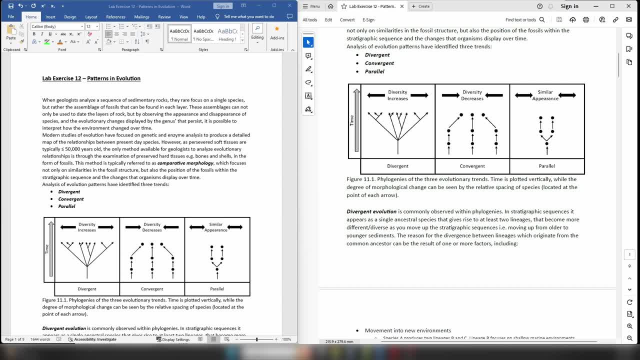 to look and see how they have changed throughout the evolution of that sequence of sedimentary rocks. So typically when we think about analysing fossils, you instantly think about: well, we'll just look at one fossil and we'll use that to date the entire sequence, or at least a. 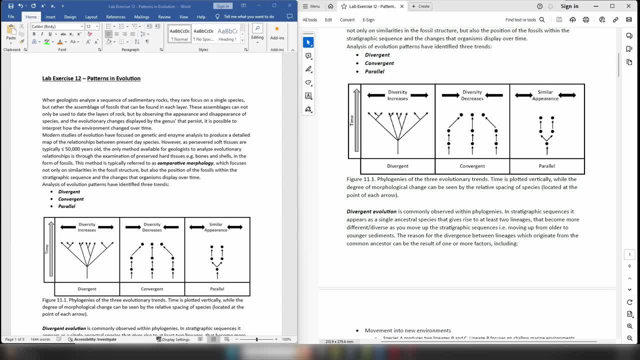 portion of the sequence. In reality, though, it's more typical for a geologist to use the fossil assemblage for each layer to, you know, gain information about that layer. So by using the assemblage of fossils, it allows the geologist to date that layer in a more refined fashion. So if you imagine, you have fossil A and fossil. 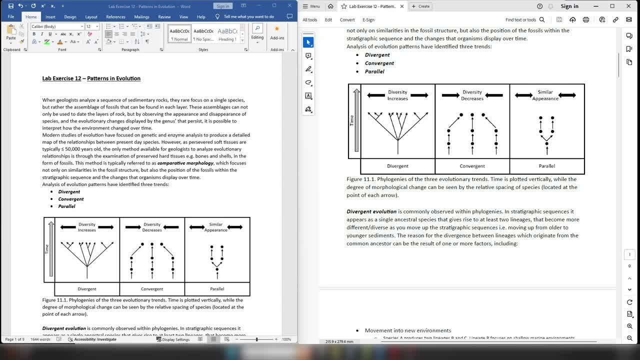 A has a range of 2 million years. And so let's say fossil A existed between 400 million years ago and 398 million years ago. So you find fossil A in your layer of rock. you say, right, well, this layer of rock clearly formed between 400 million years ago and 308 million years. 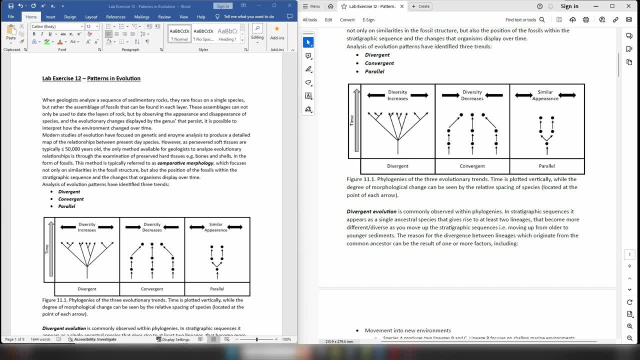 and 398 million years ago. That's a two million year window. That's quite a lot of time. So, by using the fossil assemblage, what you can do is you can locate the period of the geologic timescale when these fossils will have coexisted. 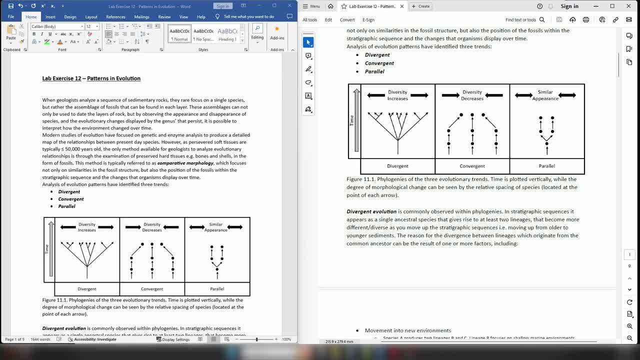 And by being selective about the fossils you choose, you can actually tighten up that dating window for the layer of rock. So using more than one fossil is typically the best choice when dating a layer. Now another thing you can do is obviously you can use 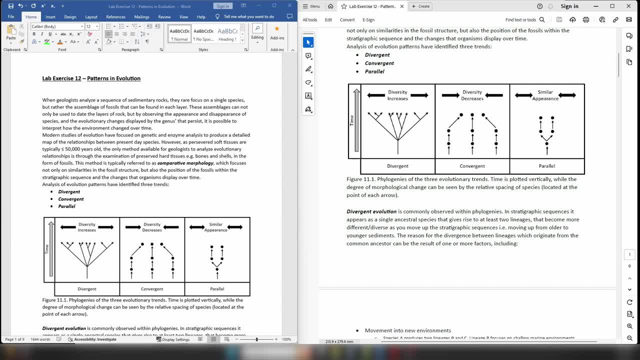 the appearance and disappearance of species and the evolutionary changes that you see as you progress up through the layers, And this is going to give you information about how the environment was changing over time, because obviously evolution is going to adapt the organisms present based on the environment. 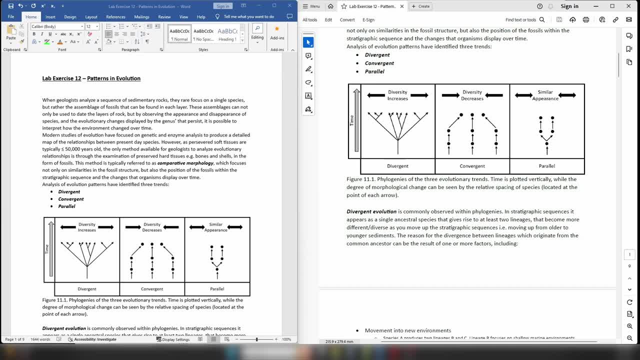 So, for instance, if you see a species disappearing, that would obviously suggest the environment is no longer suitable for them. If you see a species appearing out of nowhere, clearly the environment now suits them. And if you see changes with species that persist throughout the sequence. 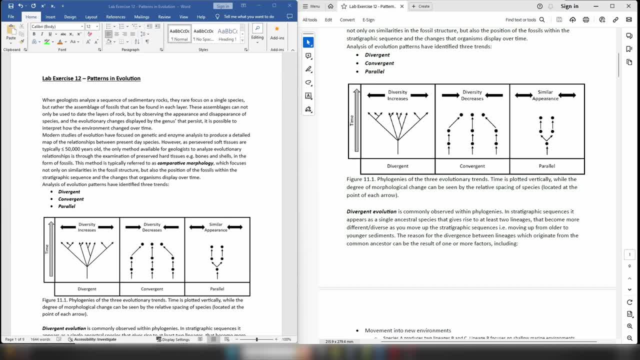 well, that's giving you some information about what's changing in the environment. So, for instance, you could start off in the lower layers with sea urchins that have relatively thin shells And then, as you progress up through the sequence, the sea urchin shells might start getting thicker. 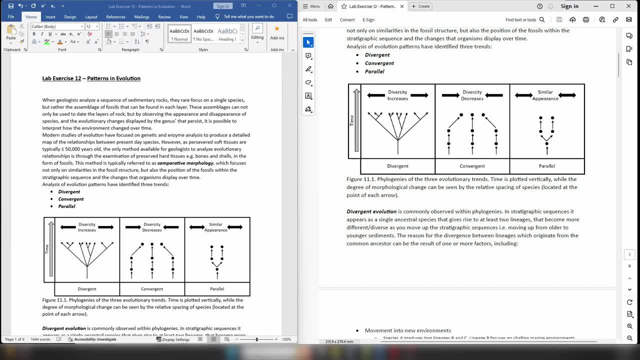 and then eventually they might develop spines, which would suggest that there's a high rate of predation. And so this is causing the fossils, this is causing the organisms, sorry to begin to come up with new defensive strategies. So when we are analyzing organisms in a modern environment, 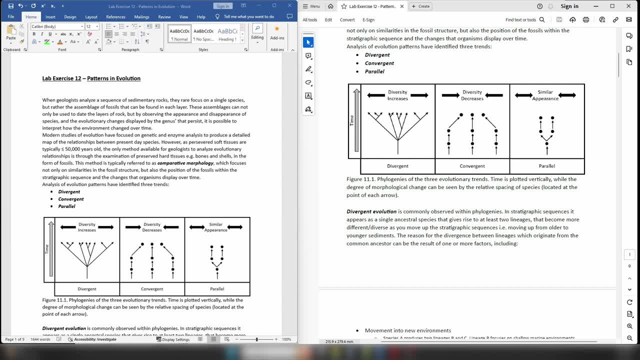 we tend to focus on genetic studies and enzyme analysis. So obviously this is exactly as it sounds. We compare DNA between species and we look for the number of similarities. Typically, the greater the number of similarities, the more closely related the organisms are. 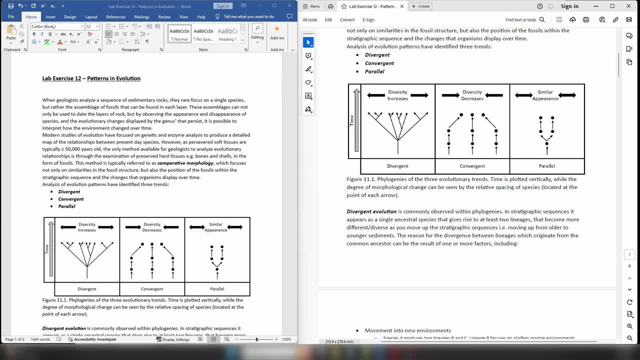 And the same things go for enzymes. so, for instance, let's just think of something like digestive enzymes. The more digestive enzymes two organisms share, the more closely related they are. The fewer enzymes they share, the more distantly related they are in most cases. 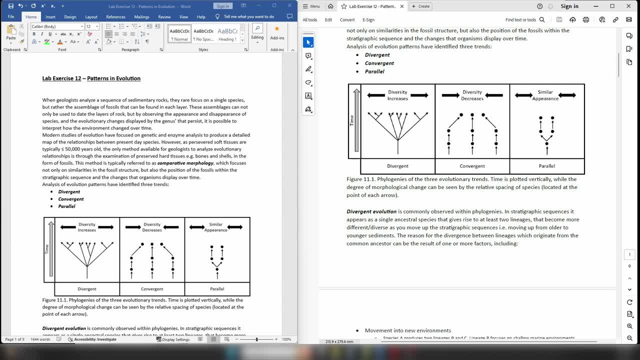 So this obviously relies on the use of the soft body parts to do this analysis. However, in geology we don't have that option because in the majority of cases, it's only material that's less than 50,000 years old where we have any hope of there being. you know, 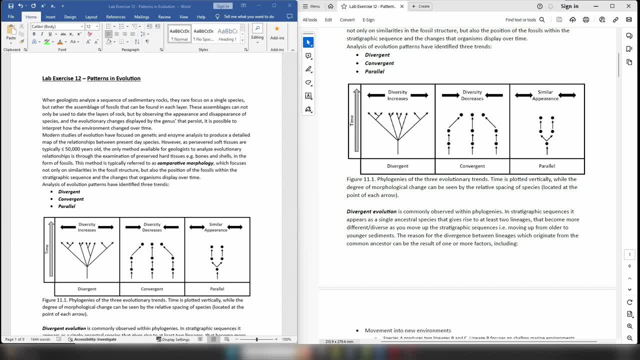 being any kind of soft tissue preserved, And even then it's typically quite a rare event. So when geologists are analyzing the fossils in a sequence, they are typically looking at the hard tissues which have been preserved as part of the fossilization process. 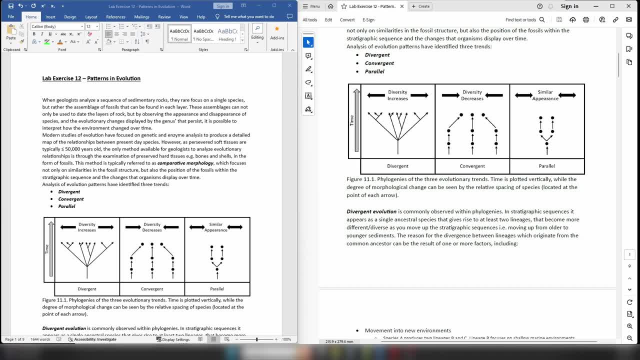 So we're looking at endoskeletons, so internal skeletons, so that's obviously, you know, animals like humans, fish, dogs, for instance. And we're also looking at exoskeletons, so that's animals like oysters, insects and arachnids. 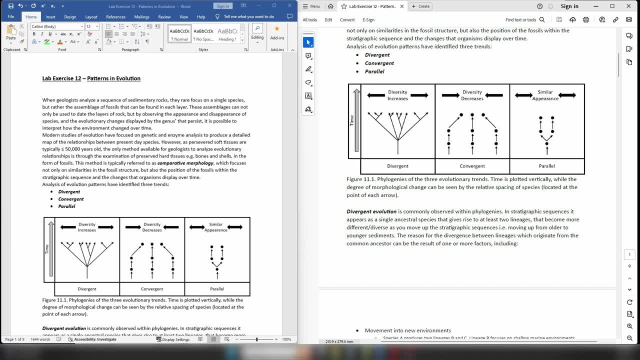 And so what geologists will do is they will compare the hard tissue and they will try and see how it's changing throughout time. So they'll compare the species in one layer to the species in the next layer and the species in the next layer. 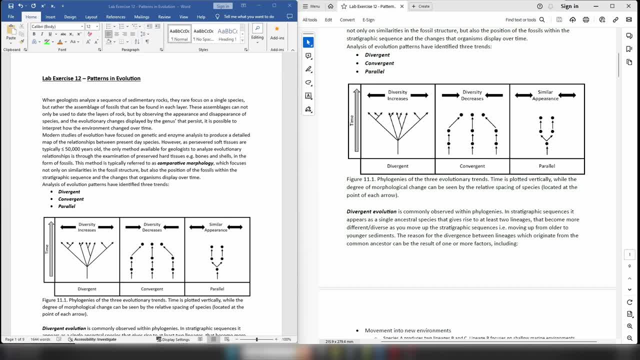 And this is referred to as comparative morphology. So they're comparing the morphology of the fossils as you progress up through the sequence and they're keeping track of the changes. Comparative morphology essentially focuses on the similarities in the fossil structure, Typically the more closely related two organisms are. 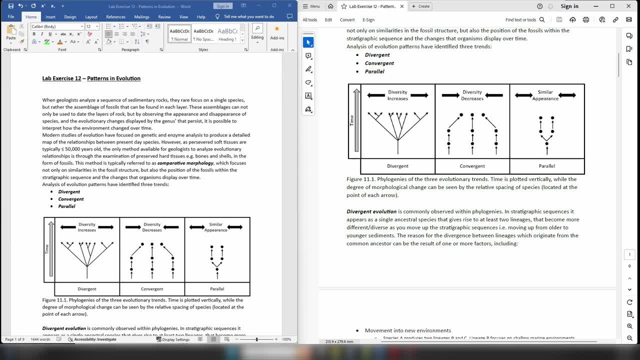 the more similarities they will share And it will also look at the position of the fossil within the stratigraphic sequence. So you know, you know, typically as you go up through the sequence, the layers of rock are getting younger. So by tracking those changes, 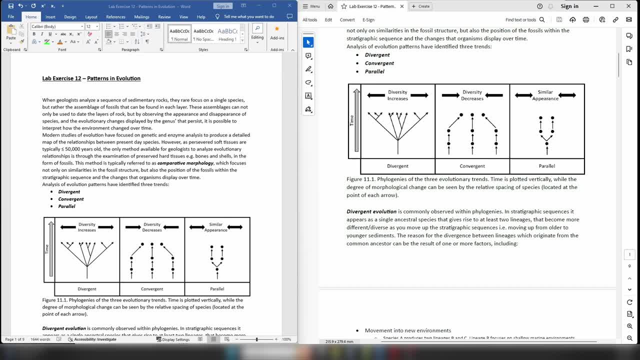 you can see how the fossil is changing as you move closer towards the present day, And so that will also, therefore, allow you to look and see how the organism is changing over time. So, by doing this analysis, what we're really doing is we are analysing. 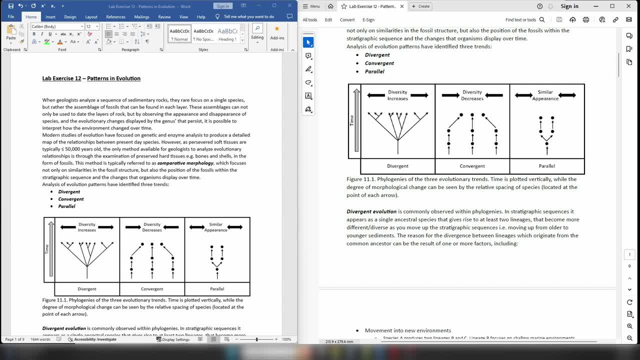 the evolutionary changes that are occurring with, you know, within that fossil assemblage which is part of that sedimentary sequence during that period of geologic time. So this kind of analysis and tracking how these changes occur throughout the fossil record has allowed us to come up with three different ways. 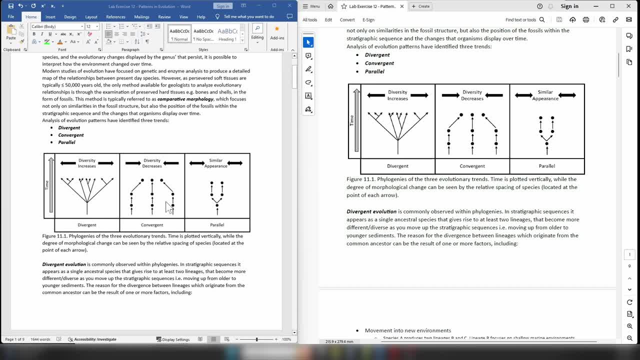 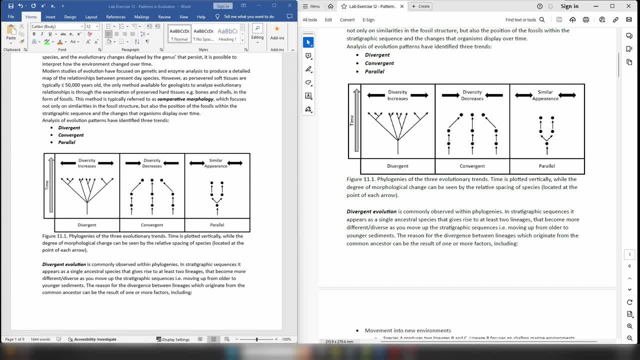 So divergent evolution is very commonly observed within the fossil record And it's defined as a single ancestor species giving rise to multiple distinct lineages. So what does this actually mean? Well, it means that, through evolution, your ancestors, your ancestors, are going to give rise to at least two distinct lineages. 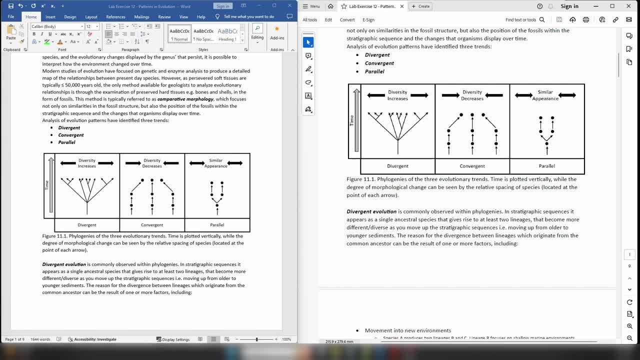 So a classic example would be something like the fish amphibian hybrids. Well, they eventually give rise to two distinct lineages, the amphibians and the reptiles, And then both of those lineages will then diversify even further. So the amphibians will diversify. 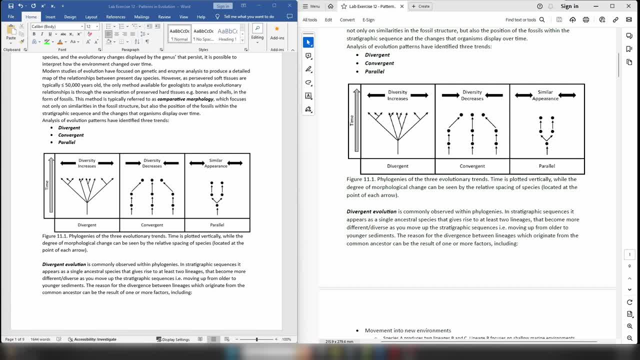 into multiple different types of amphibian and the reptiles will then diversify into distinct groups of reptiles- so crocodiles and alligators, turtles and so on. And the reptiles will then diversify into distinct groups of reptiles- so crocodiles and alligators, turtles and so on. 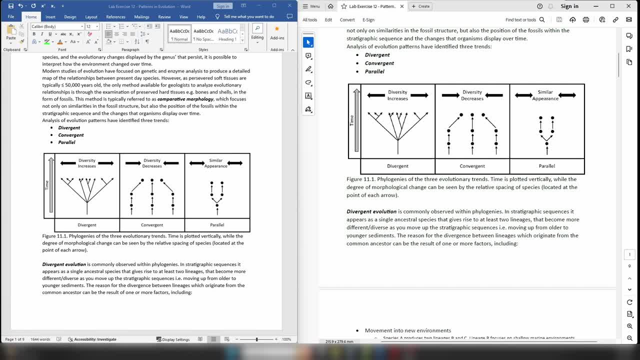 And then the reptiles will then diversify into distinct groups of reptiles, so crocodiles and alligators, turtles and so on. Then obviously, further on from that, we'll then see the reptiles diversifying to birds, And obviously we'll then see the reptiles diversify. 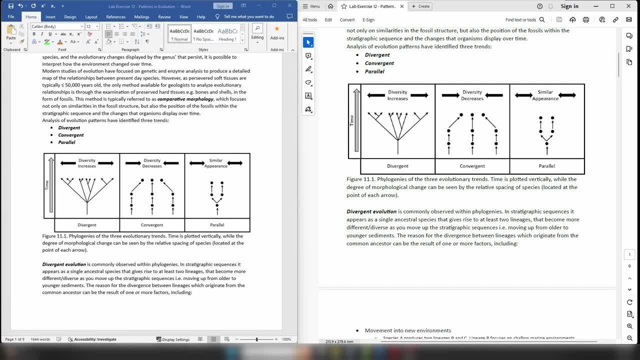 to give rise to mammals, And then the mammals will then produce multiple different lineages as well, And so this pattern of evolution is going to produce this tree-like structure. So, as you move up through your sedimentary sequence, you're going to start with your ancestor species. 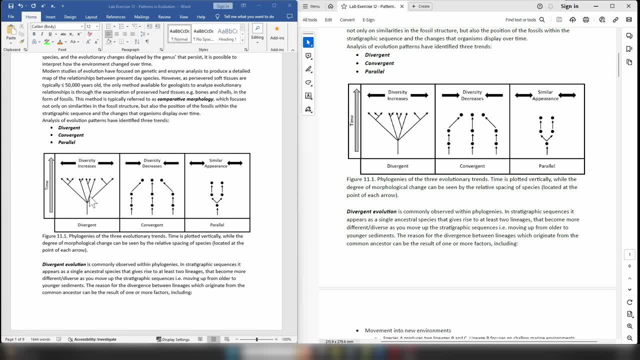 in the bottom layer And then, as you move up, layer by layer, you are going to see the ancestors of that individual, of that ancestor species, becoming more and more diversified, becoming more and more different and becoming more and more specialized to whatever type of environmental niche. 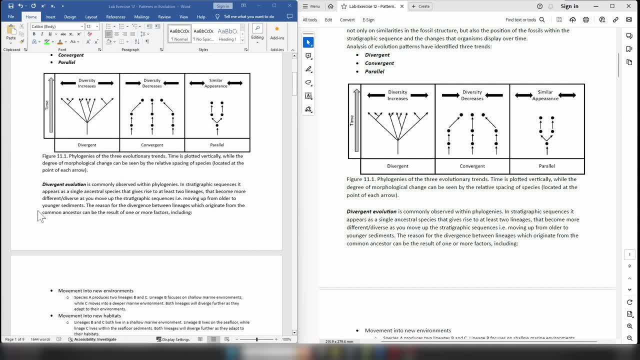 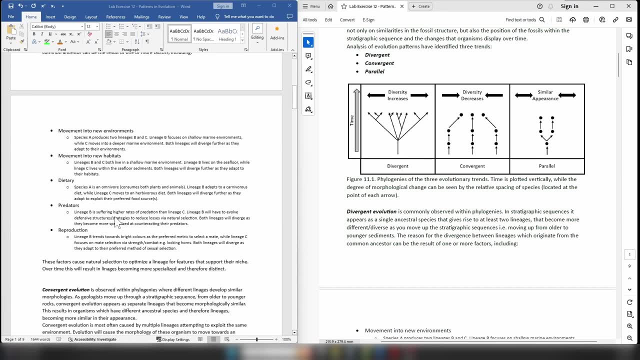 they are trying to exploit. so, when we think about divergent evolution, what are the driving factors behind it? so why are we actually seeing this ancestral species and the lineages that come off it diversifying and changing so much? well, obviously there has to be a factor which is: 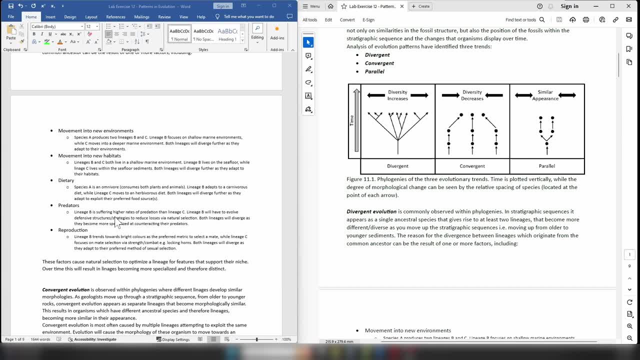 encouraging this change to happen, because under normal circumstances, if there is no reason for evolution to take place, it typically won't. so one of the more common reasons that you can see evolution occurring is if you have an organism that is moving into a new environment, so in this instance you would have, for instance, species a. 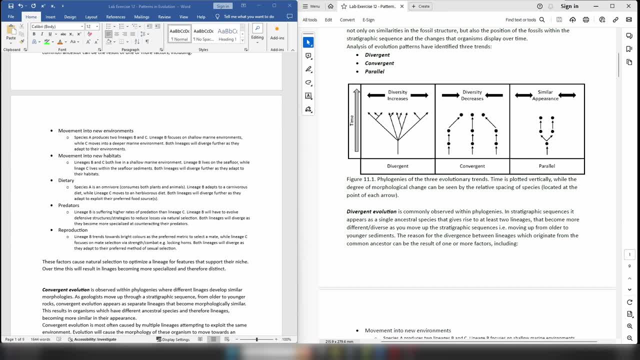 and species. a is the ancestor to species and it's going to give rise to two new lineages, B and C. So in this instance, lineage B is going to focus on a shallow marine environment, whereas lineage C is going to start exploiting maybe slightly deeper marine environments, and so obviously you're going to see both of these. 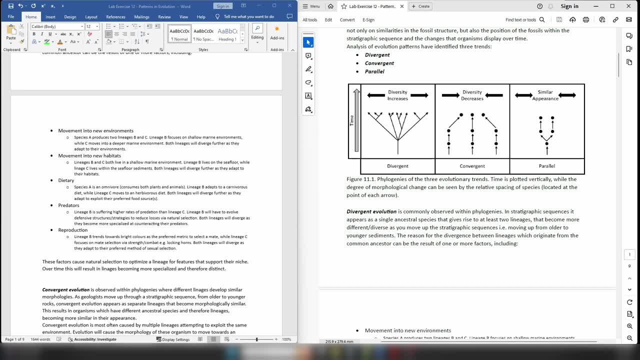 lineages beginning to diversify as they adapt to these two distinct environments. So another situation is: maybe you have a situation where you have the new lineages moving into new habitats. So once again, ancestral species A gives rise to lineages B and C, and both of these lineages, B and 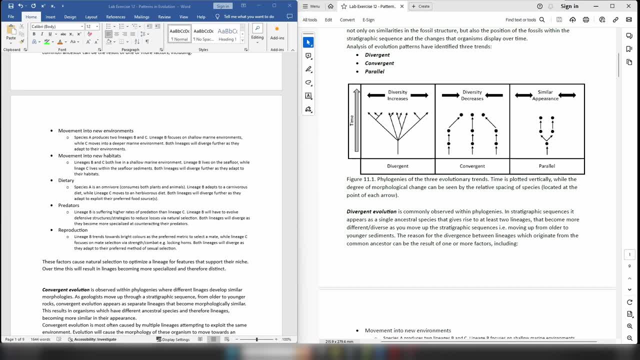 C are currently in a shallow marine environment. So lineage B is going to live on the seafloor, while lineage C is going to start to exploit the seafloor sediment environment. So it's going below the surface into the seafloor sediments. Once again, what you're going to see is you're going. 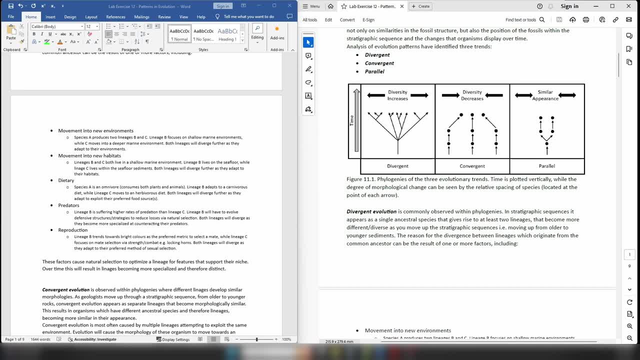 to see the lineages diverging. So, for instance, lineage B might develop defensive structures associated with protecting themselves from predators. because they're on the seafloor, they're exposed. In contrast, lineage C will not develop similar structures because they are in the sediment, which gives them a certain amount of protection and having additional protection. 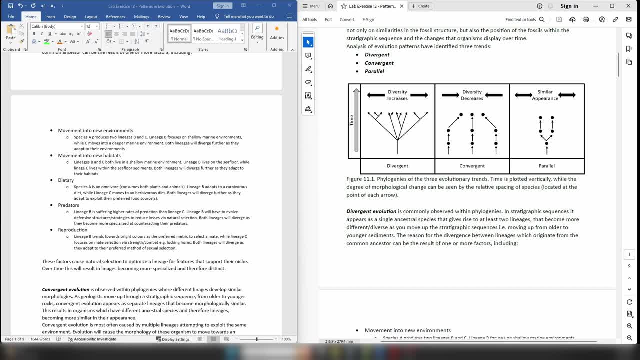 like spines for instance, will actually inhibit their ability to move through the sediment and get away from predators. So you can see how these two lineages are going to start diverging and they are going to begin specializing for their distinct habitats and changing to accommodate them. So another factor which may cause evolutionary change is a dietary change. 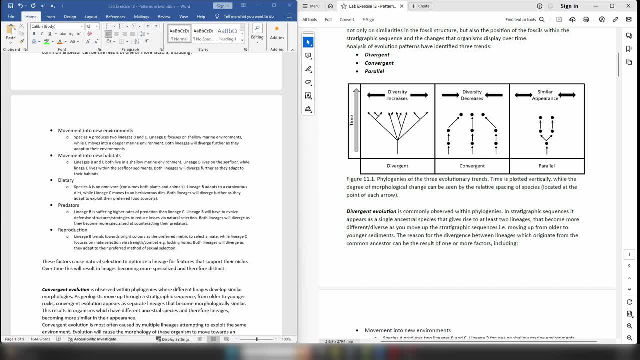 So let's say once again: we have our ancestor species A and they are going to produce lineages B and C. So for ancestor species A, let's say it's an omnivore, so it's consuming both plants and animals. However, maybe lineage B begins to move to a more plant-based diet or maybe a more meat-based diet. 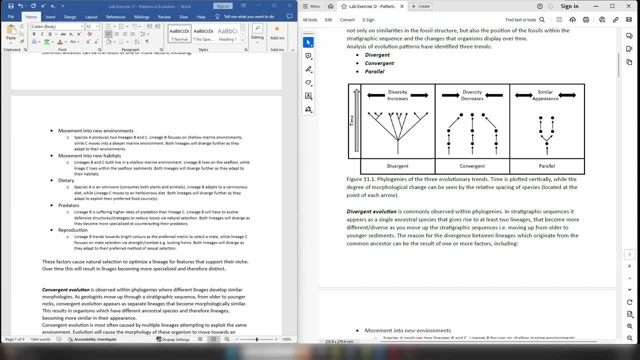 So in this case, let's say, lineage B becomes carnivorous and it starts to focus exclusively on eating meat, while lineage C becomes herbivorous and it will start to focus on eating plants. Obviously, once again, because of these dietary differences, you're going to see these two. 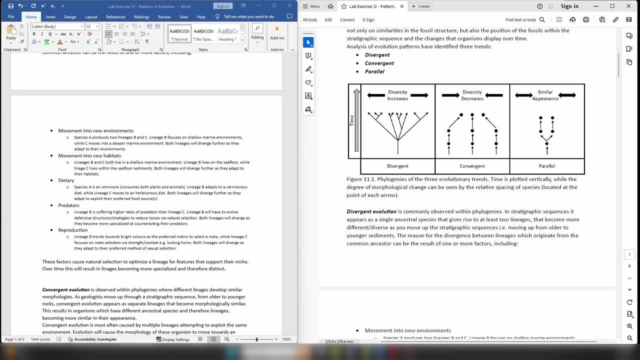 lineages begin to diverge from one another and become more diverse. So the herbivorous lineage will then start to exploit more and new different types of plants, so you'll get even more diversification, Whereas the lineage B, which is now carnivorous, that's going to start focusing. 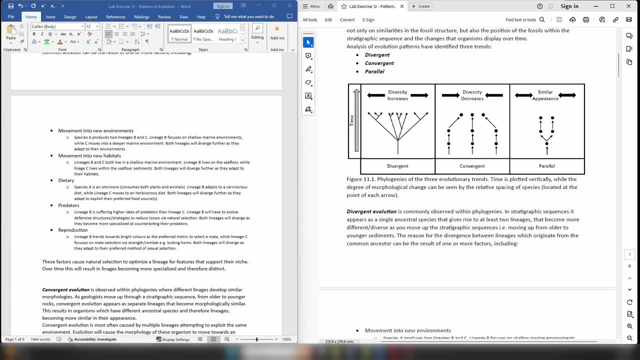 on different ways of attacking their prey. So it's going to start specializing based on what kind of prey it's going after and it's also going to start specializing in how it will attack that particular type of prey. So, once again, from this ancestor species we get this radiating effect where we 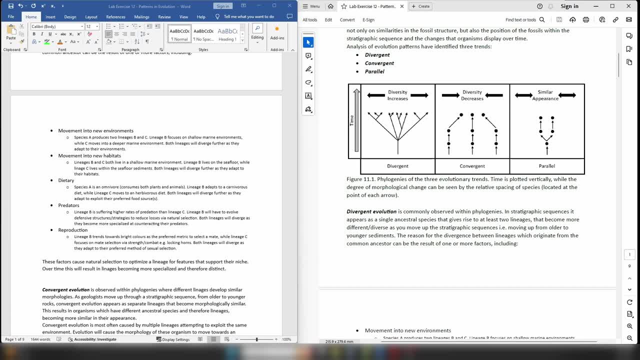 have more and more diverse descendants. So another driving force is predation. So once again we have ancestral species A. it's giving rise to lineages B and C. If lineage B is suffering a higher rate of predation than lineage C, then lineage B is going to have to try and evolve defensive structures or strategies. 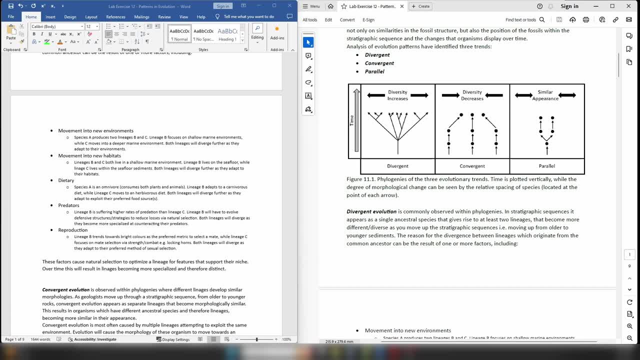 to reduce losses, And this is going to occur through natural selection. So, obviously, organisms in lineage B that do not have predation are going to have to have predation. So if you do not have a good strategy, are going to be picked off and become extinct, Whereas organisms that do. 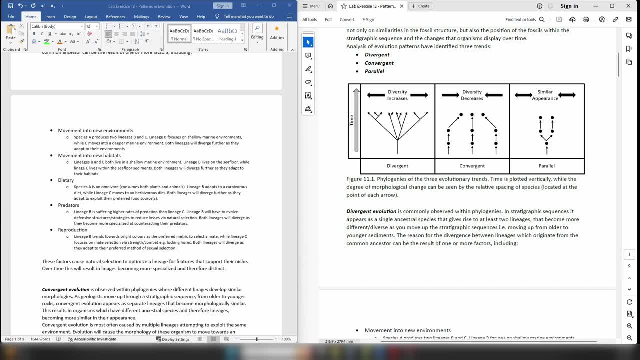 have a good strategy to survive, will be less likely to be killed off, And so you will see that species begin to dominate that lineage, and then, obviously, those particular traits will then be shared throughout a diverse group of descendants. Now, obviously, both of the lineages will show: 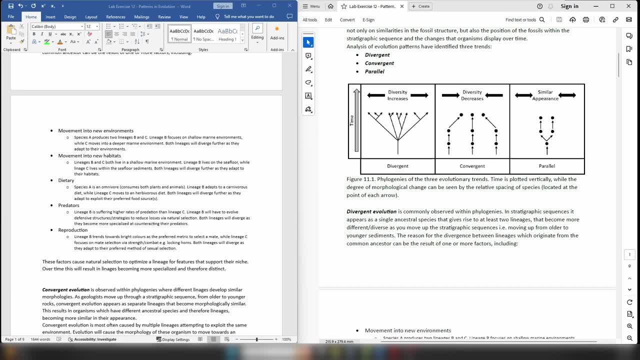 diversification to avoid predators, because they're both being preyed upon. But in the case of lineage B, what you would observe is you would see these changes associated with predation occurring faster than for lineage C. The final thing that could be driving divergent evolution. 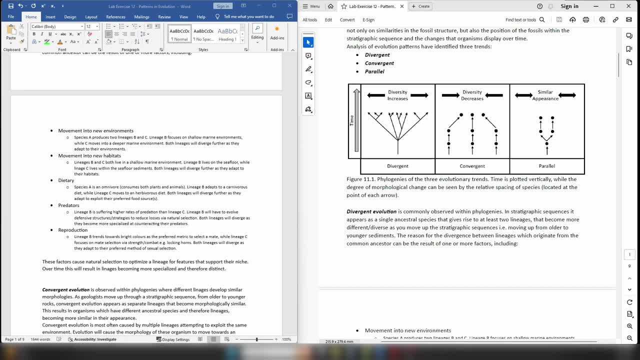 is reproduction. So in the case of reproduction, you have ancestral species. A is giving rise to lineages B and C: Shock horror. So lineages B and C, let's say lineage B, trends towards using bright colors as predation, One of the metrics which is used to attract mates, While lineage C maybe focuses on a mate selection. 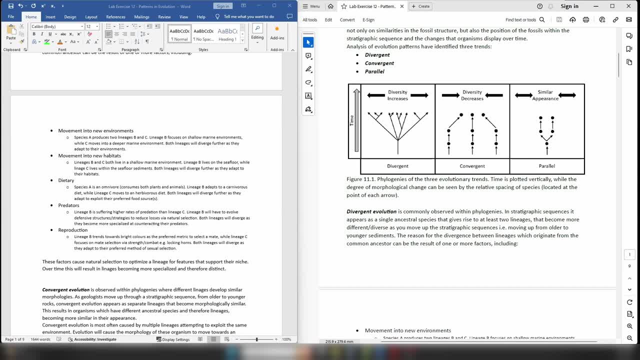 via some kind of strength or combat based event, For instance locking horns. So obviously you are going to see both of these lineages diverge as they adapt to their preferred method of sexual selection. So you'll see, maybe lineage B will become, you know, have developed even brighter. 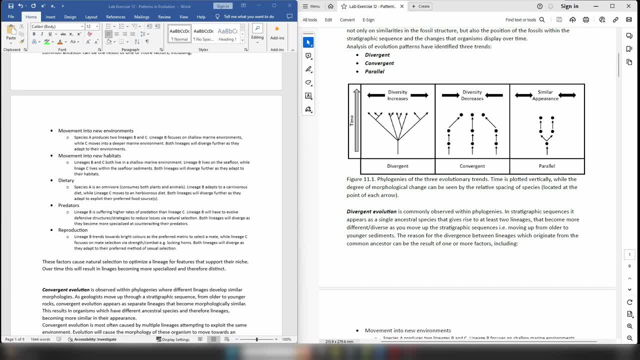 colors and more impressive displays to try and attract more mates- successfully. Whereas in the case of lineage C, maybe you will see that particular lineage will develop into organisms with stronger neck muscles, maybe bigger horns, more robustly built skulls, for instance, And so all of these pressures 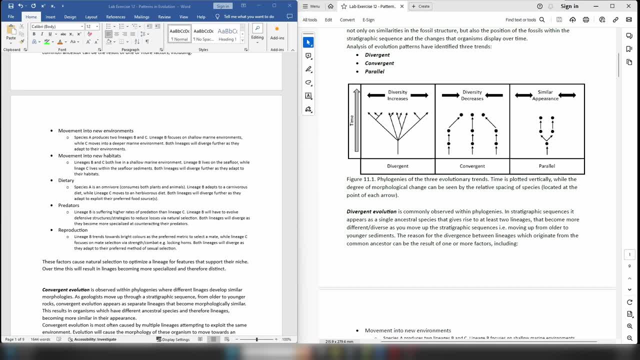 often working simultaneously, will drive the diversification of species over time, and it will mean you'll end up with lots of diverse descendants which have you know. if you trace the family tree back, you will see they have all come from one shared ancestor species, And so when we analyze the 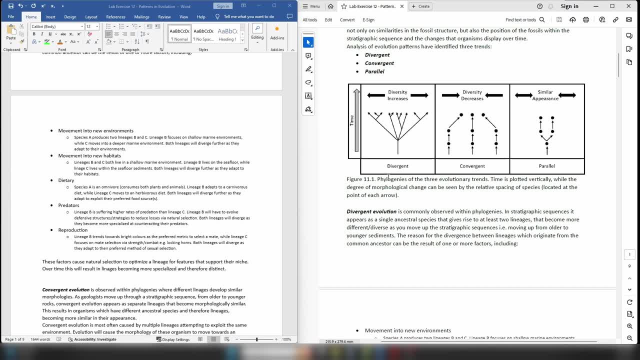 changes in the fossils. as we move up through the rock record, we will see this tree like structure, where we have the ancestor species down at the bottom here giving rise to these multiple and diverse branches which become more and more complex over time. So the second pattern of evolution observed in the fossil record is convergent evolution, And this is 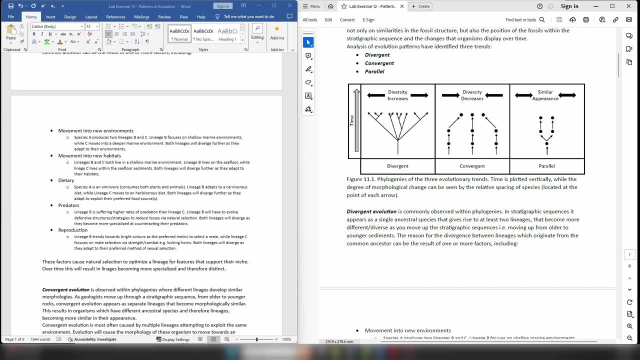 observed within phylogenesis. Phylogenesis is when different species have different genomes. So if you go over here, if you scroll down here, if you scroll down to the left, we will see there are different species of genomes from one generation to the next. And in Lost Rock region, where different 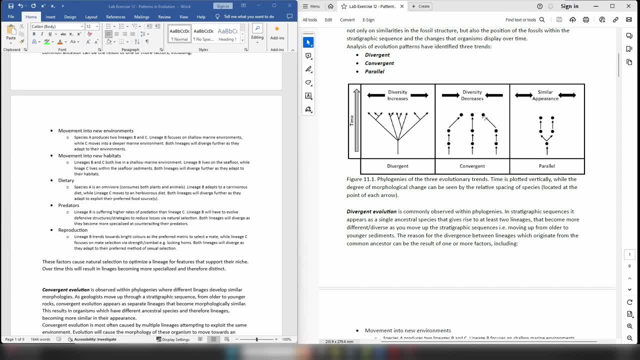 species have the same genomes, so these three species are the ones that are the most diverse in this region. Now, if we go back over here, we will have the following case, where a number of species are divided up into different groups. So we will see that the top row is a couple. of species, But this is where we can see they really have different genomes and we can see that the top row is a group of species, But in the bottom row we have a group of species where different species are completely different to one another, So we'll notice a decrease in diversity. 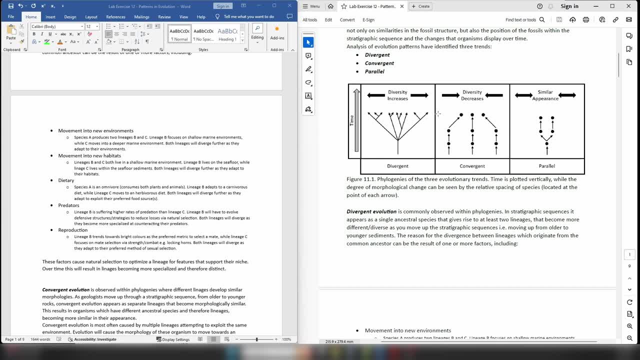 So we will see these three lineages will begin to show morphological similarities And we obviously younger layers. So convergent evolution is most often caused by multiple lineages attempting to exploit the same environment. So obviously, for each environment there's going to be a set of 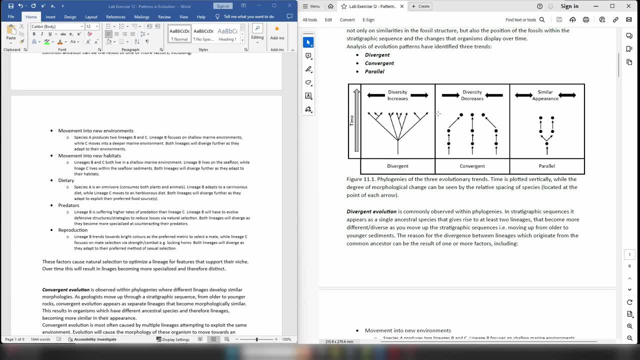 optimum body designs for that particular instance, and so it's not unsurprising that different lineages will begin to show a similar morphology as they all begin to adapt towards these better morphologies for the environment in which they are living. So the classic example of this is: 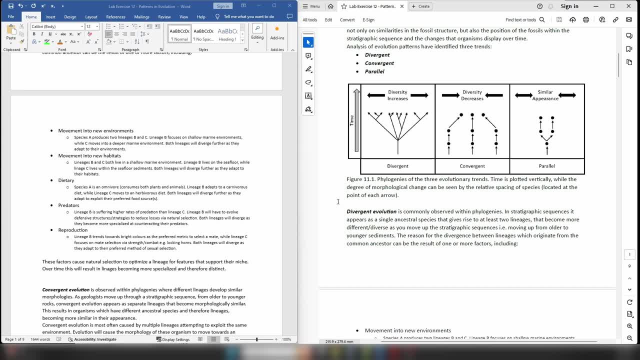 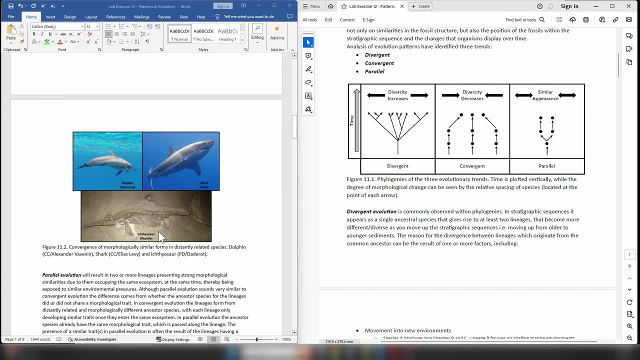 sharks, dolphins and ichthyosaurs. So if I just yeah, so obviously we have dolphins, mammals, sharks, fish and ichthyosaurs, which are reptiles. However, you will notice that they do share a lot of similarities. So they've all developed conical heads. they all have long, smooth bodies. they 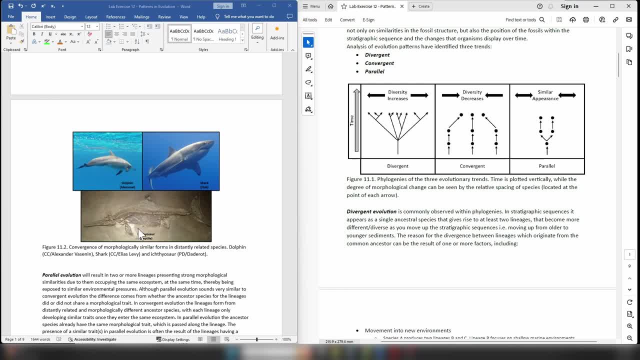 have a lot of hair. they all have a lot of hair. they all have a lot of hair. they all have a lot large pectoral. so front fins for steering. they have a dorsal fin for stability when turning and a powerful flute tail for propulsion. And the reason they all show very similar body. 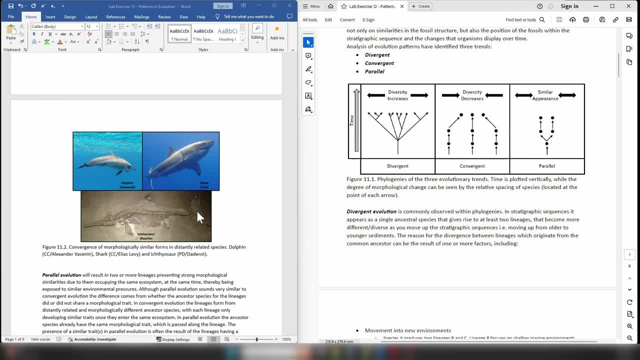 morphologies is simply because this is one of the most optimal designs for a predator in the marine environment. So it's not surprising that as this mammalian lineage and as this fish based lineage and as this reptile based lineage began to move into the marine environment. 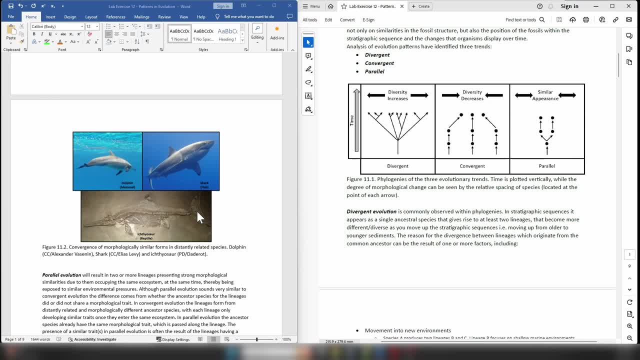 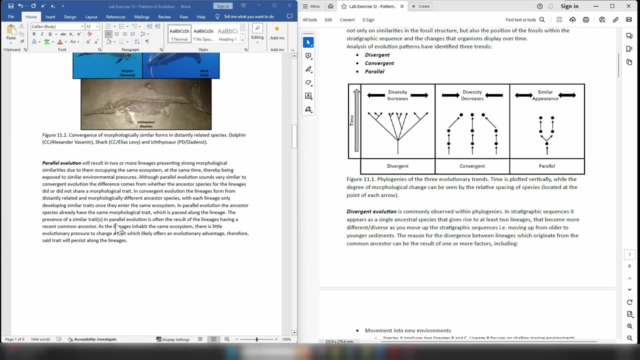 they began to develop a similar body morphology because it's exactly what was needed to become, you know, for their optimum survivability. So the final type of evolution which is commonly observed in the fossil record is parallel evolution, And this will result in two or more. 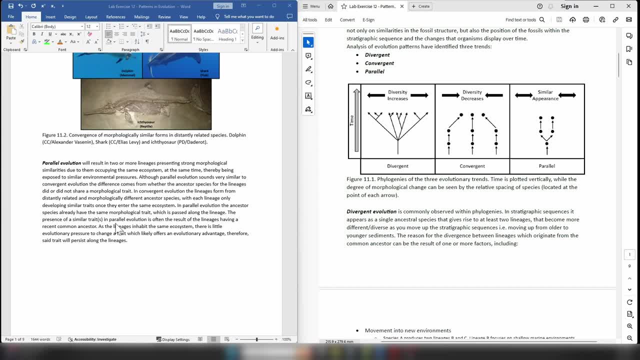 lineages presenting strong morphological similarities, and they will typically be occupying the same ecosystem. So once again, we have a situation where we have this optimum body design for that particular ecosystem. So these organisms will be occupying the ecosystem at the same time and they are therefore being exposed. 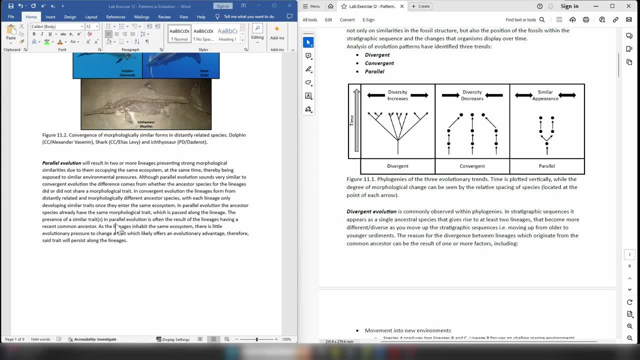 to similar environmental pressures, which will, you know, encourage natural selection to select the same advantageous traits. Now, parallel evolution does sound very similar to convergent evolution. however, the difference comes from whether the ancestor species for the lineages did or did not share a morphological trait. 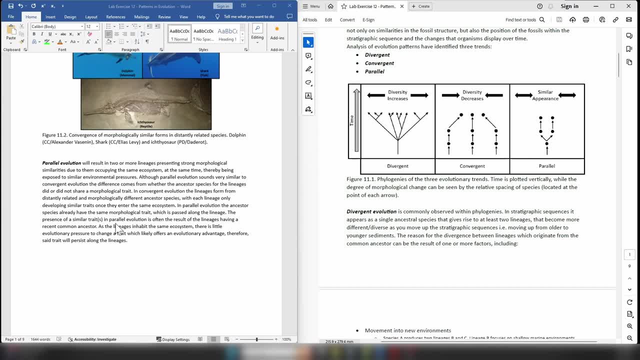 So in convergent evolution, the lineages form from distantly related and morphologically distinct ancestor species. So you have pre-lineages which are very, very different from one another, and each of those lineages begins to show morphological similarities in response to the environment. 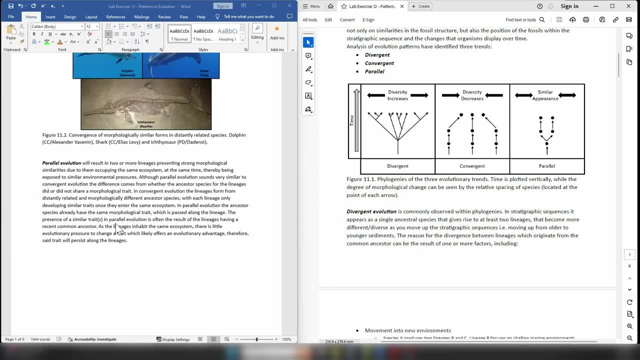 Now, in the case of parallel evolution, what you're dealing with is that these organisms have an ancestor species that already have the same morphological trait. So both of these lineages are essentially coming from a recent ancestor species that they both share, and so that common trait, which is advantageous- 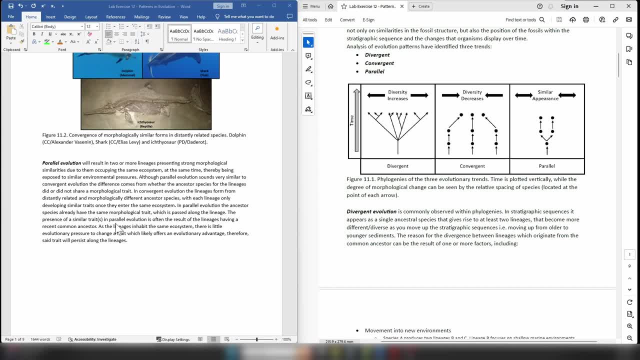 for that environment is then maintained by the two lineages that form from the ancestor species. Now, if we look at the second lineages, the ancestor species is usually the same as the morphological trait. the reason this particular trait persists is because it is the most advantageous trait for 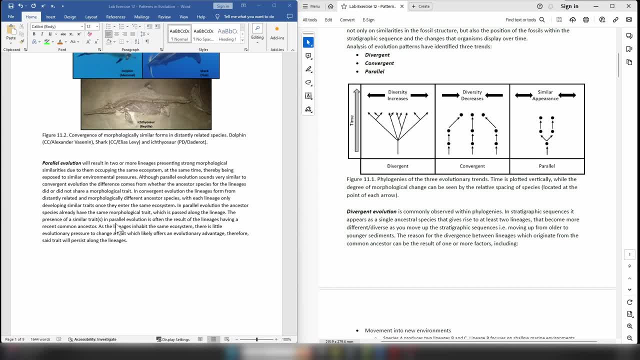 that environment, so natural selection isn't going to try and get rid of it. instead, that trait will persist over time and will be carried forward in each iteration along that lineage, and so the classic example of this is, of course, mammoths and mastodons all essentially share a common ancestor. 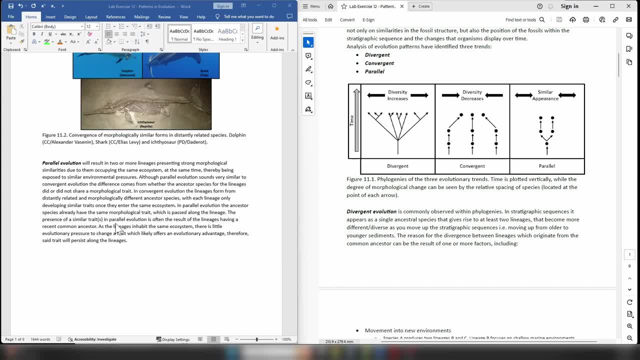 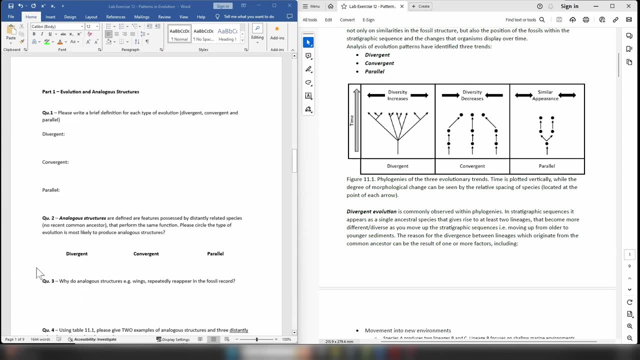 and all show very similar morphological designs based on the type of you know, because they share relatively similar environments. so that would be the classic example of parallel evolution. okay, so I think that's it for part one of this video, so please get up have a walk around. 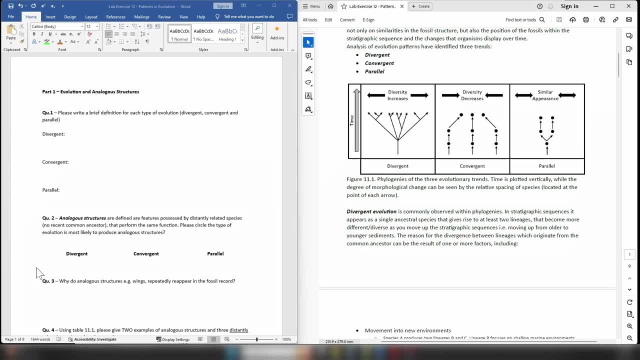 get a glass of water and then come back for part two. 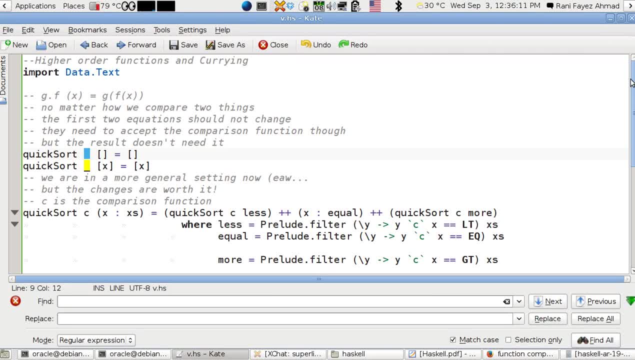 hello hi, this is Rani Ahmed with you and this is lesson 19 and how to program using high-skill programming language, and this is I'm going to talk about higher order functions and carrying now in this lesson, I have to go a little bit from.